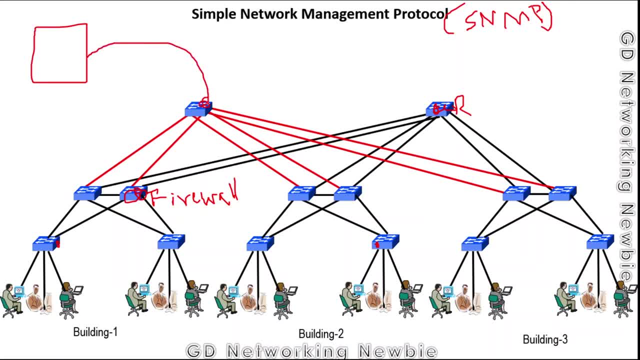 where we want to monitor all these devices, We want to manage all these devices. Maybe we want to maybe troubleshoot these all devices if there is any problem in the network. So for that purpose, for monitoring the performance, to troubleshoot the network, we needed a protocol, we needed 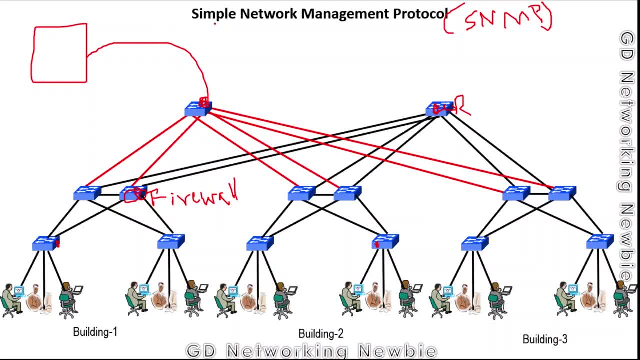 some rules and now those set of rules are thought. That protocol is SNMP, So let's remove this first. So SNMP is a protocol which works at the application layer And this is a protocol which is used for management and the monitoring of networking devices which we have on our network. So SNMP can be used. 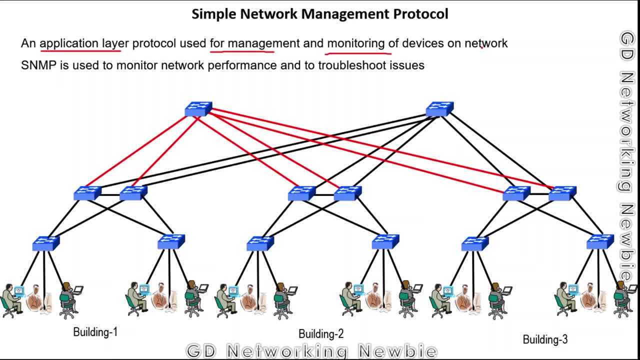 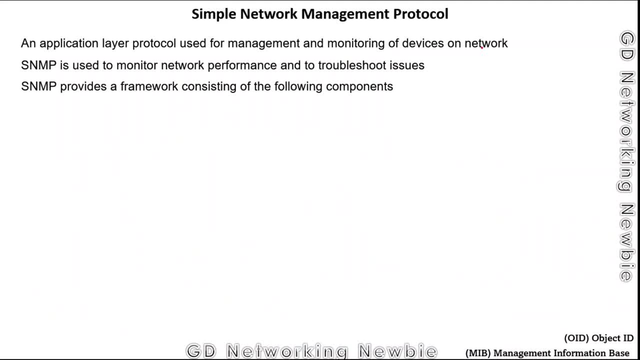 to monitor network performance and to troubleshoot issues. Now this SNMP provides a framework. In that framework, we have the following components. The first component is the SNP manager. So SNP manager is a network management application. We have a server, We have a PC here. We have a server, We install the relevant required. 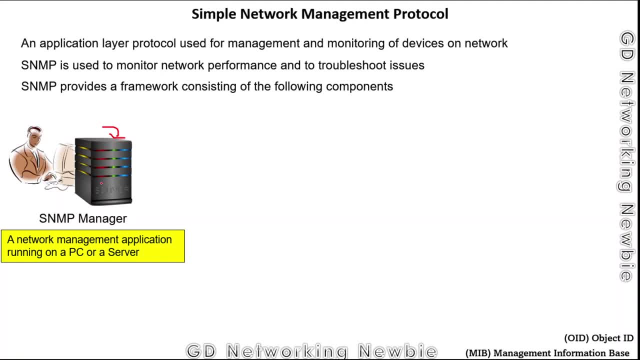 application there And this becomes SNP manager And this host is known as network management station. So this is the first component. This is the SNP manager, from where we want to manage our network. And now these are the devices It needs to be monitored And those are known as SNP agents. So in this SNP framework we have the SNP manager. 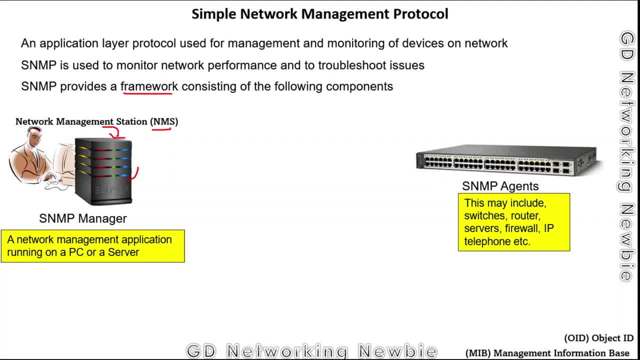 and we have the SNP agents, And these SNP agents may include switches, routers, servers, firewalls, IP phones, So these all can have as an SNP agent. It needs to be monitored by some, maybe network administration. So that's why we have the SNP manager here, And those are all the devices there We want. 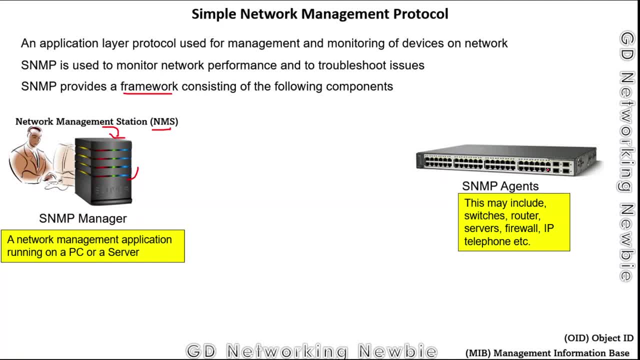 to monitor them. So this is the second entity and on these devices we have some database and that database actually is stored. that database is known as management information base, that is MIB management information base, And in that management information base we have some specific database. 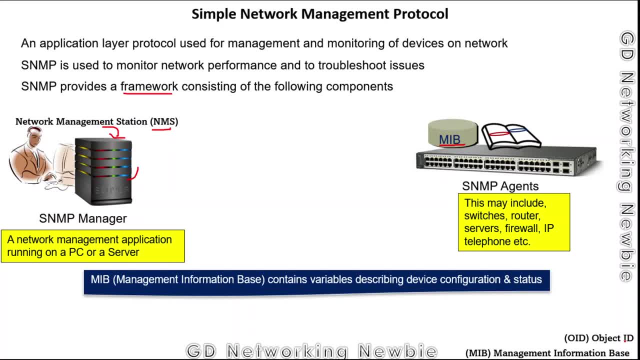 that needs to be monitored. Okay, variables, and those variables are describing the device configurations or device status. so let's say this device is running. on this device we have maybe different interfaces: gigabit Ethernet, fast, fast Ethernet interface. then there are multiple variables which actually define the operation of this networking. 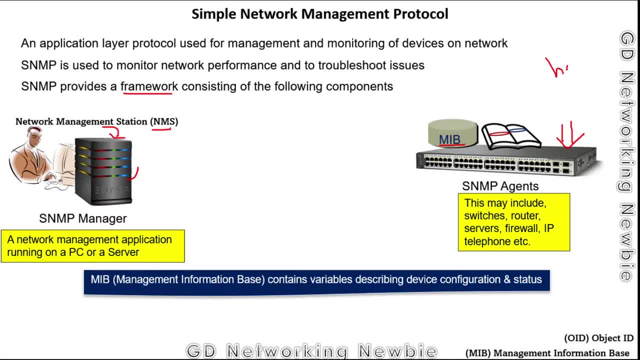 device, like the hostname itself. so this device will have a name, hostname, so that hostname will also be saved in a variable as a variable in this management information base. so all these things are available in a form of variable on these S&P agents. and now, yeah, so these variables, these variables. 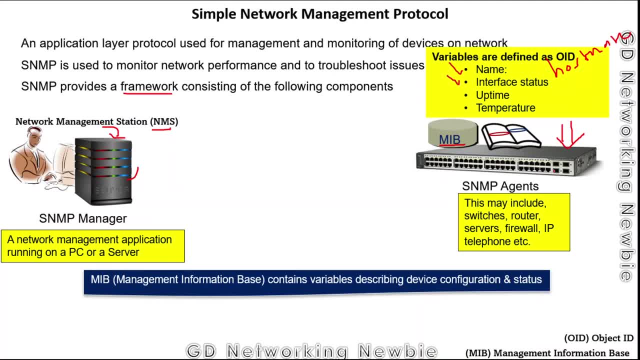 can be named. these variables can be interface status- like we can have multiple interfaces- whether that is interface is working properly or it's not working, or what is the uptime for that interface, what is the temperature, for instance, in some of the devices? so these are some of the things which we want to monitor and those and 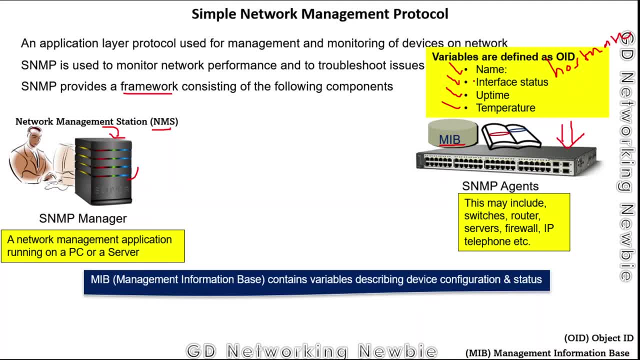 those things are are known as variables, and those variables are defined as OID. so OID stands for object ID, by which we refer, and to these all variables. okay, so now we have the variables which are showing this status of these devices and we have the S&P manager from where we want to manage. 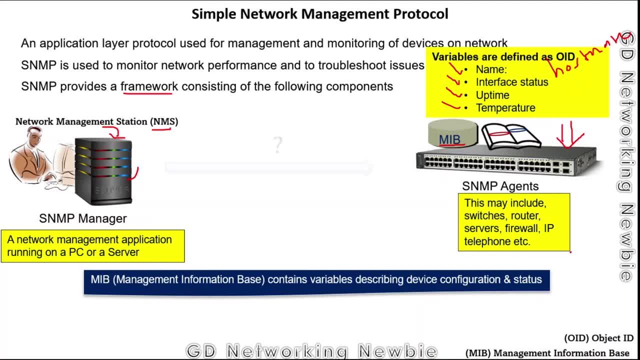 or observe these devices. now this protocol. so these are three elements here. so S&P manager, first element. S&P agent, second elements, and this management information base. this is the third element. and now this protocol. S&P protocol provides a way by which we can exchange this information, which is available in this management information base. we can 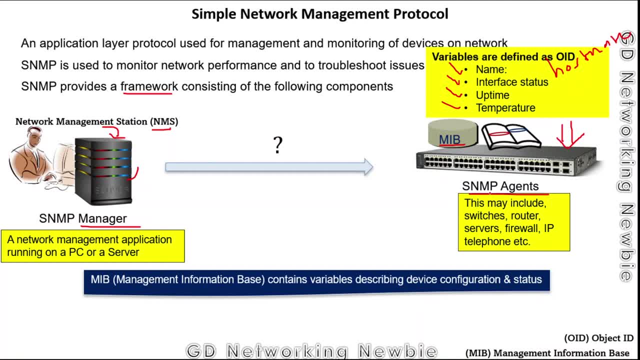 exchange this information between S&P manager and the S&P agents, which are basically our devices. so in this case this S&P manager can actually send a query message to this device that please send me the status of some of the interface, maybe fast Ethernet interface. send me the status whether that is the. 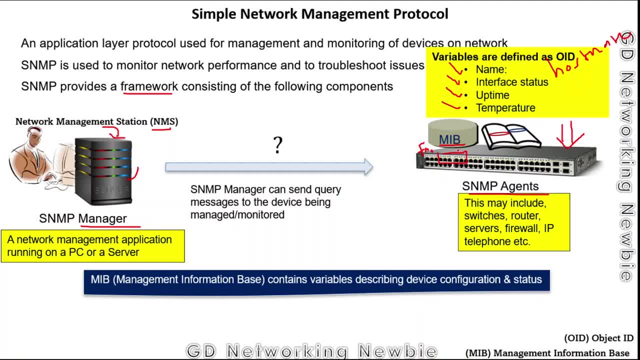 interface is working or not and the status of that interface will be saved in some of these variables. and now the those variables will be sent to the S&P manager and on the S&P manager we will have a screen here and on that screen this network administrator actually can see whether that particular interface is. 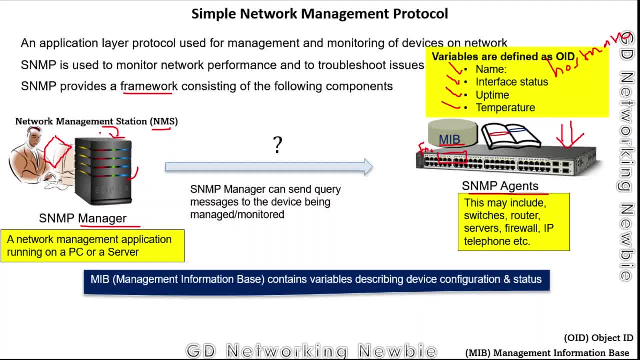 working or not. so by sitting at the remote and somewhere else we can monitor the interface and like, and these all are the variables which we can access. so S&P manager can send a query message to the device being managed or monitor. so these are the device which can be managed. okay, and for this, for sending the request. 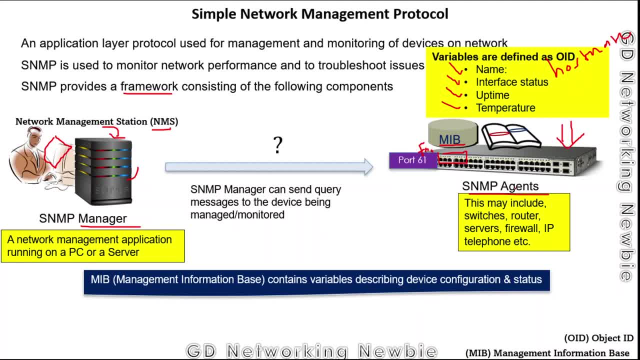 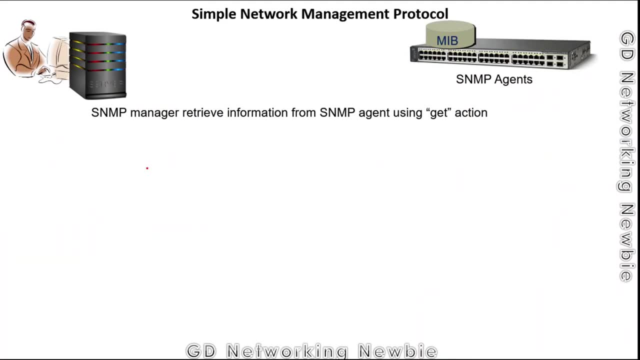 port number 61 is used at this end at the S&P agents end, and when we are receiving that information at S&P manager, then port number 62 is used and we will be sending a query message to the S&P agent and finally use UDP at the 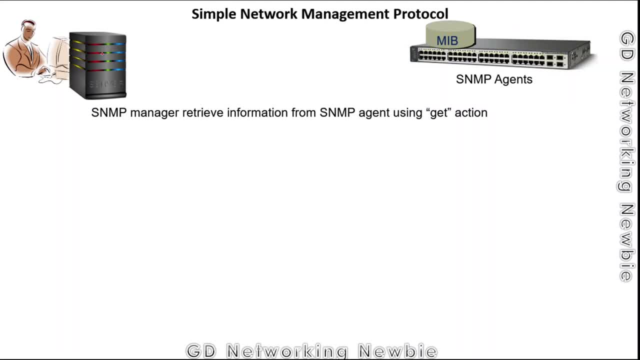 transport layer. so we discuss that. on S&P agents, we have some set of variables and those set of variables can be accessed from S&P manager and for that S&P manager uses some actions. so an S&P manager can retrieve the information from S&P agents using get action, get action here and with this. so let's say we have a 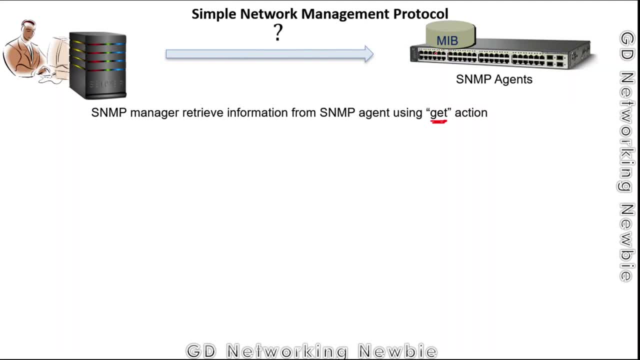 Let's say, please send me your name, Please send me the status of some of the interface, for example, Please send me the uptime, for example, So these all information can be retrieved from this management information base using get action. and as a response, this snp agent will send back the. 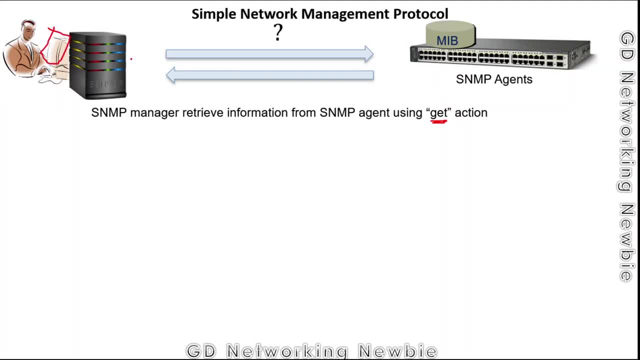 required information to this snp manager to see this information and in this get, for example, they can ask for the device name, they can ask for the interface status, they can ask for the routing information. these are some of the things they can be done. there are many things there which can be. 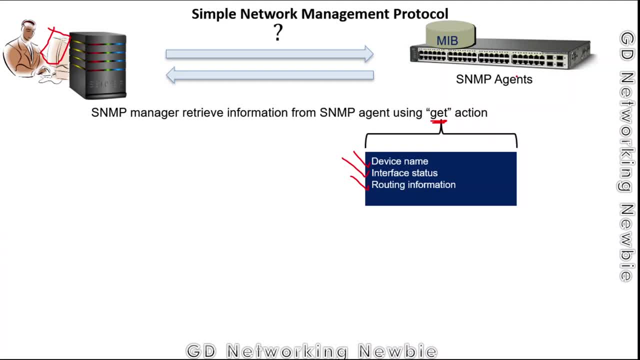 done. this depends what kind of variables are defined on this: snp agents and then this snp manager. so with the help of this snp manager we can set some of the variables here. for example, we want to change the status of some of the interface, like the status may be up or down, so we want to change the status of some. 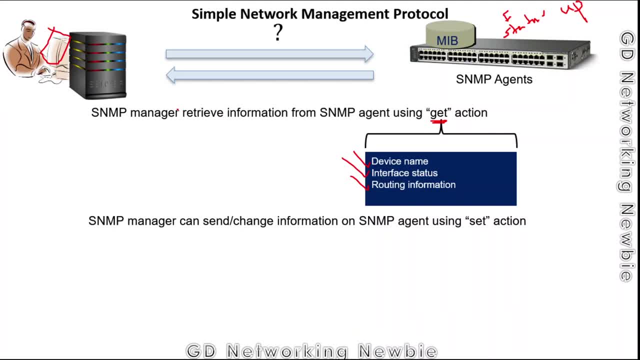 of the interface there so that can also be done with this snp manager. so in this case, snp manager can send or change the information on snp agent using set action. so we want to set the variables and those variables are defining the behavior of this networking device that is known as snp agent. 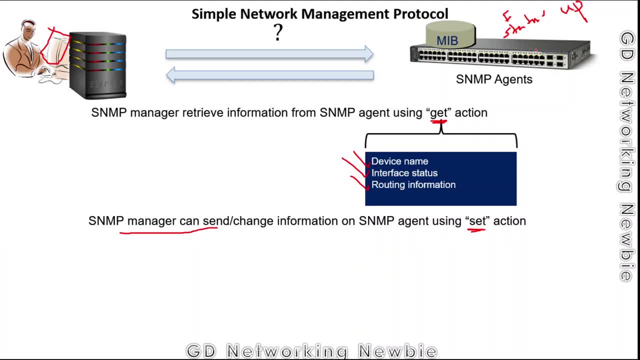 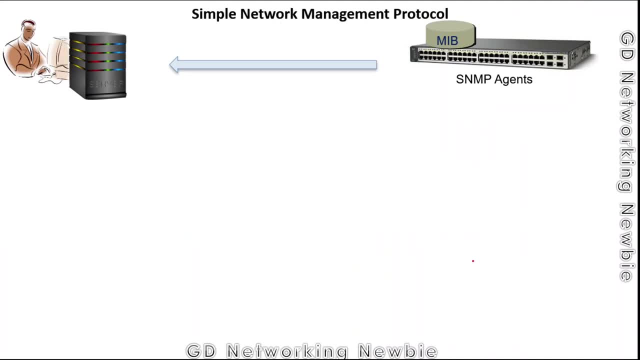 in this case. so get means we want to retrieve some information. set maybe means we want to change or we want to send some information to snp agent. so in addition to those messages, these snp agents- so in these before- i mean in the previous slide- i discussed that this snp manager is sending some requests- 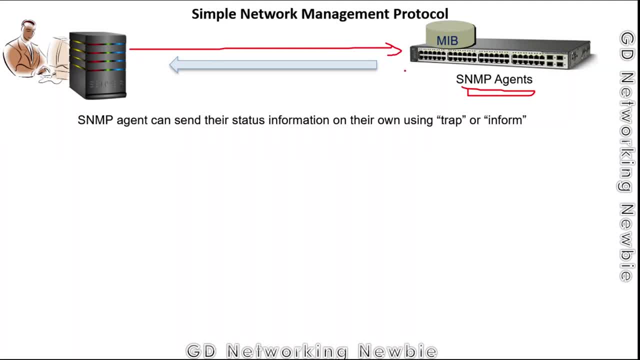 are going to pull all these devices and, as a result, of all these devices are reporting this information. it means it's going to to ask them. but let's say that there is some emergency, for example this: this switch has been rebooted or some unauthorized user is trying to access it, and this is some kind of emergency. 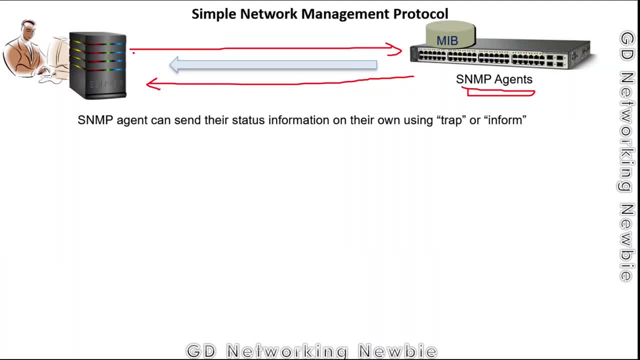 information, and this information should be sent to this snp manager as soon as possible. and that thing is also possible in simple network management protocol, and for that the snp agents can send their status information on their own, on their own, without asking, without being asked by this snp manager. so for that they use trap and 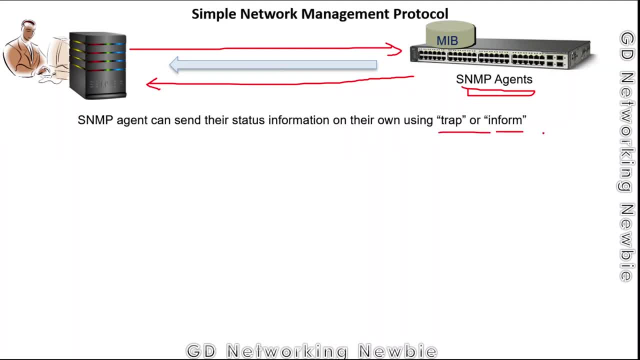 inform messages. so these are the immediate message of the urgency messages which are which are being sent to the snp manager. for this they use a trap and inform, and the difference between trap and inform is that that for informed messages, so this snp, same snp, is sending some status. 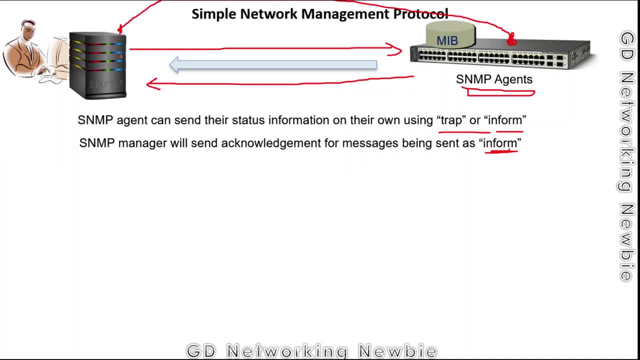 information using inform. so in that case snp manager will be sending back a feedback. but if this snp agent is sending some trap messages, so for those trap messages snp manager will not be sending back any feedback. so that is the difference in between trap and inform messages. 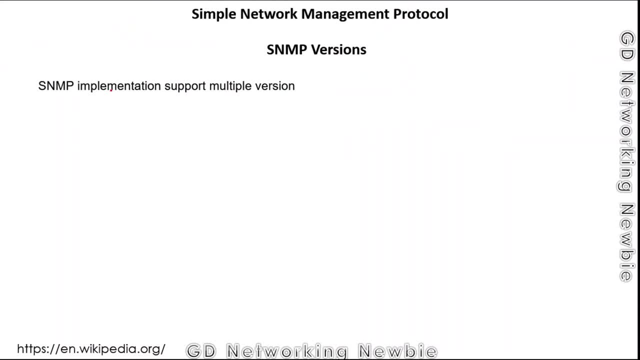 and now there are three versions of snp. the implementation support multiple versions. this is the first version, so this is, that is snpv1. this is the initial implementation of snp protocol. this is the first version, and then there is the second version, that is snpv2c. this is, uh, the improved version of snpv1 and this introduced 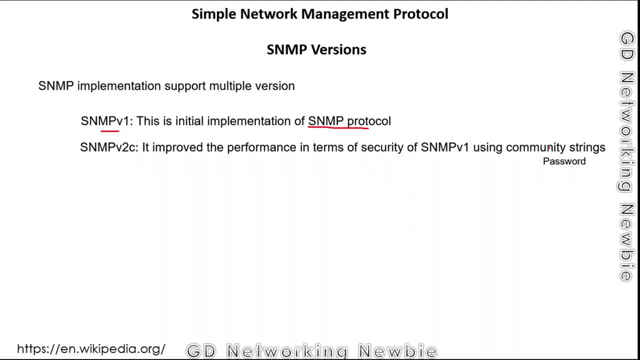 this uses the security using community strings, so that is kind of a password there. and the third, that's version three. this provided uh, confidentiality, integrity and authentication. so this is only the password in plain text. but now we have in this snpv3 confidentiality, which is provided using using encryption, so nobody, nobody else, can actually. 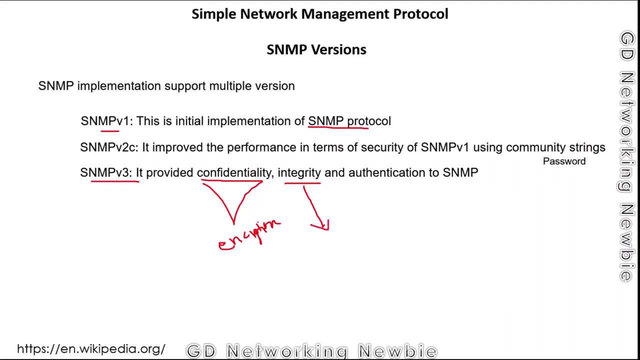 can read the message: integrity, to ensure that the message has not been changed from snp manager to snp agent or from agent to manager. so this may happen that some, some of the person, can change that message and to make sure that nobody has changed that message, we need this. 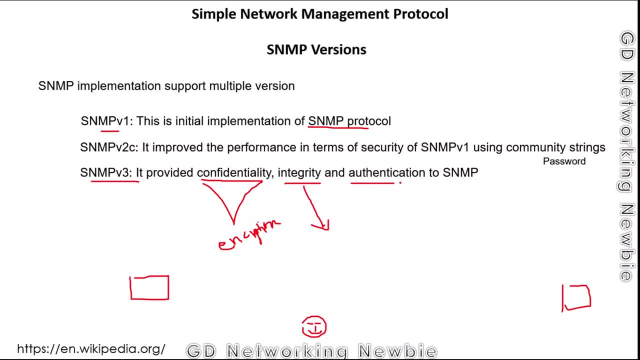 component, that is, integrity, and then also authentication, and authentication message, or authentication, is used to verify that the sender is really the legitimate sender or to verify the identity of the source. so this is the first version of snpv1 and then the second version of snpv2. 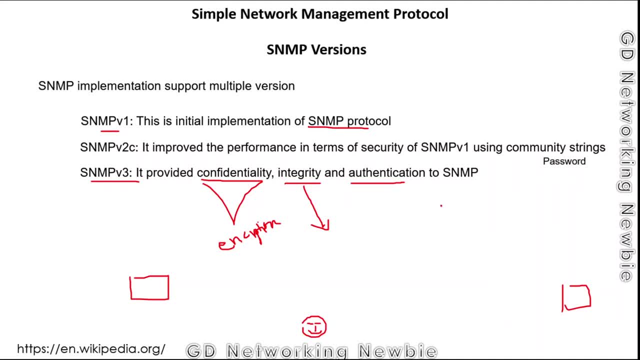 these are the important things which are provided in snpv3, and this is the end of our discussion on snp. i hope this discussion might be helpful for some of you and thank you. thank you very much for your time. hope to see you in some other video.